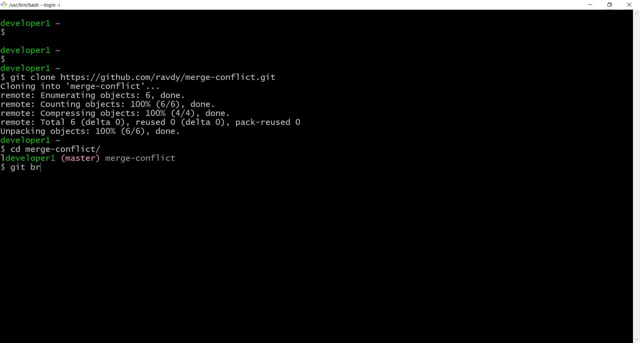 You are going to get your repository and, by default, git branch. if you check, okay, git branch. if you check, you have only one branch. that is master branch. usually developers doesn't work on the master branch. they create a new branch out of that and they do the changes over there. 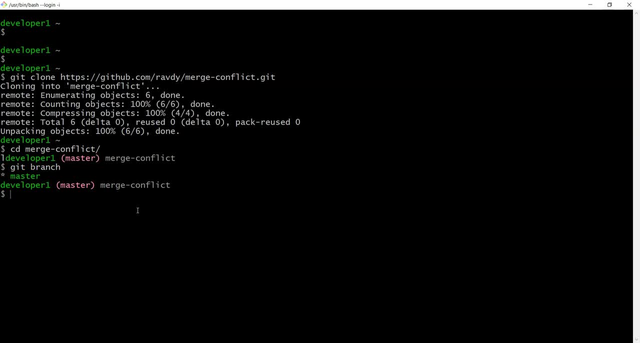 So let's take an example that I'm creating a new branch called git branch. okay, dev1 branch. okay, because it is a developer1.. So developer1 branch I'm creating. Now we have created a new branch And if you check git branch, now we have two branches. 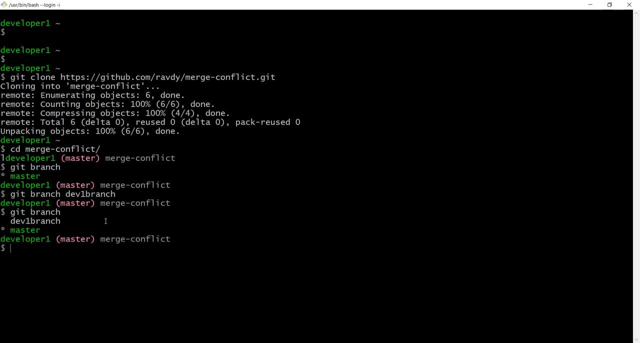 So let me switch on to dev1 branch and let me do my changes. So git checkout. git checkout is the command to check out to dev branch. So dev1 branch. All right, I have switched to dev1 branch and git branch. if I check again, okay, you can see. 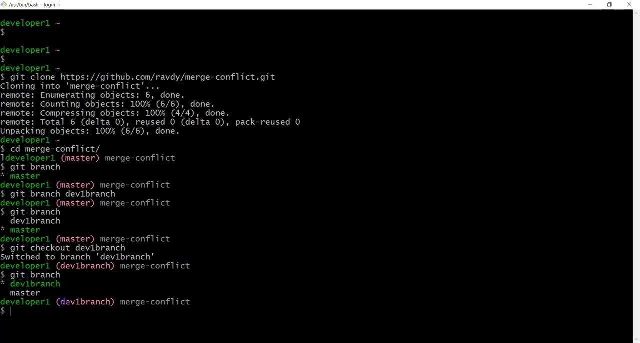 The green color and the star means you are in dev branch. of course, in my git bash I have updated so that I will get this information over here in which branch I'm working. fine, So now let me do the changes to my file. 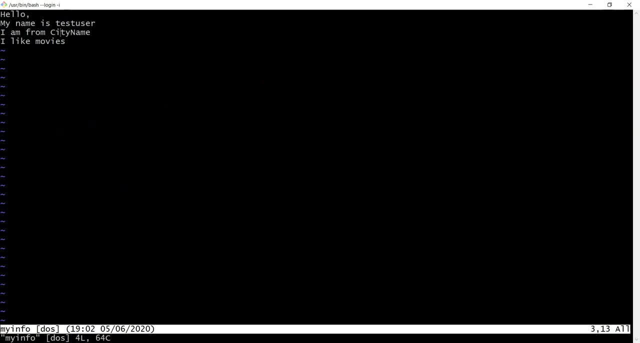 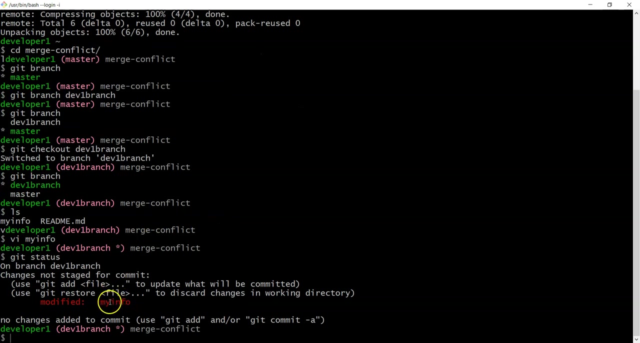 So, via my info, and here I'm going to change my username to developer1,. okay, so this is how I'm fixing this issue and I'm from Bangalore. okay, I just updated this information and git status. if I see so, I have modified my info file on the dev1 branch. 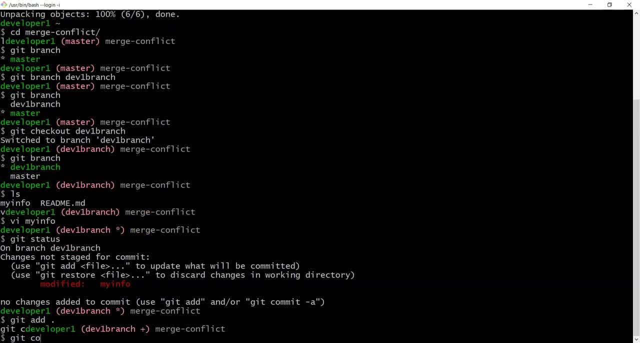 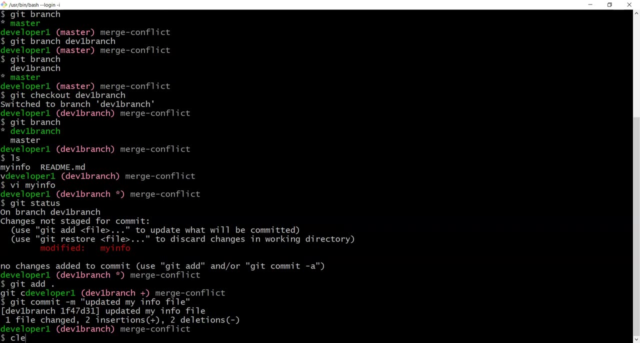 So git add dot, git commit minus. m updated my info file, okay, so I have updated or committed these changes into my local repository, not into the remote repository. So git add dot, git commit minus. m updated my info file, okay, so I have updated or committed these changes into my local repository, not into the remote repository. 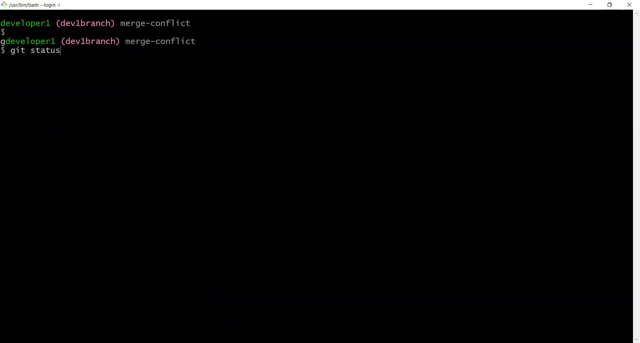 So git add dot, git commit minus. m updated my info file. okay, so I have updated or committed these changes into my local repository, not into the remote repository. Once this is done, I need to git status. So nothing is there. My branch is clean and I would like to commit these changes to the master branch. 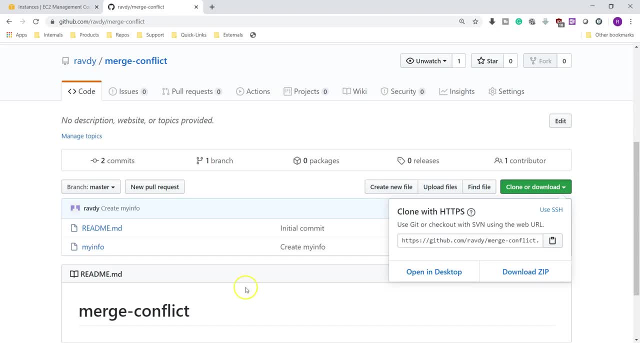 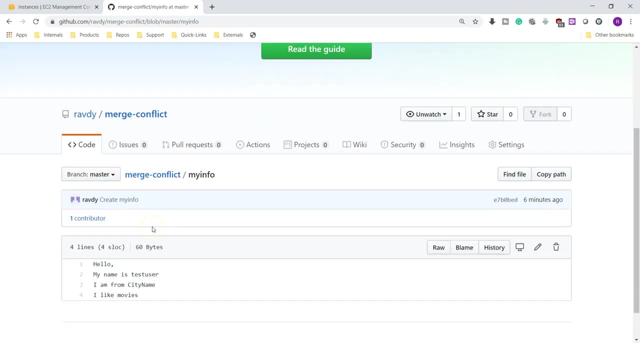 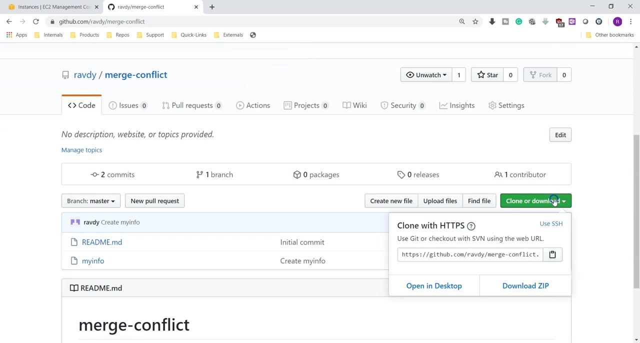 Okay, But meantime one more developer has seen this code and even he thinks that, okay, this is not in the right format And if you see here, it is still not yet committed as a developer one, So you can still see the same code. and he thinks that, okay, let me correct the bug. 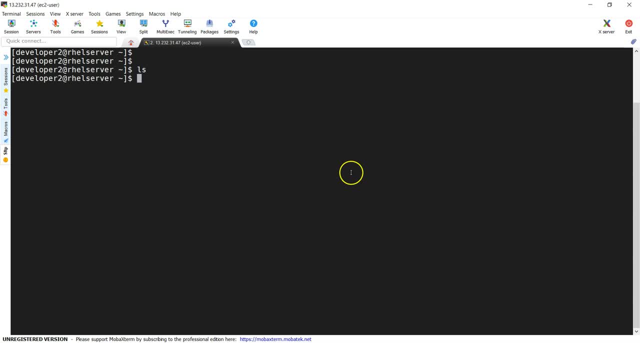 So what? Okay, So what? So what he is doing? he is also cloning this repository onto his system. So, git, clone, I'm cloning this repository And if I see I have merge conflict repository and he went inside and he would like to commit these changes. 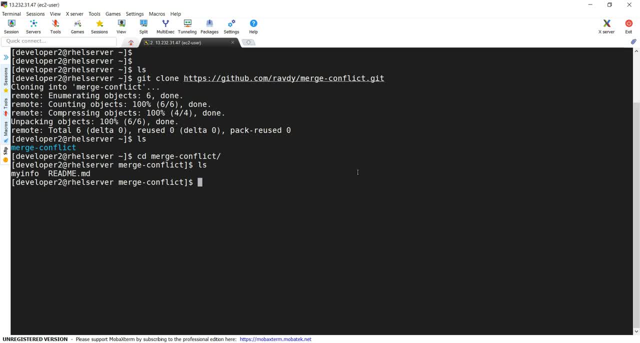 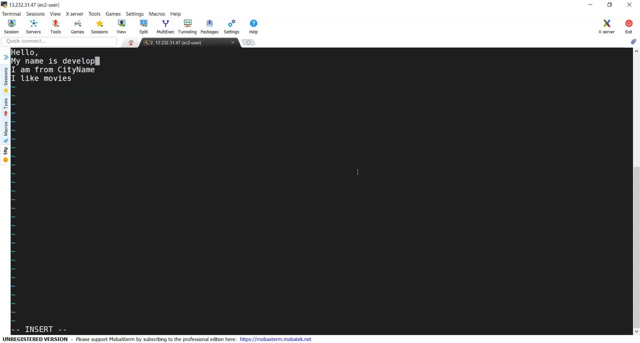 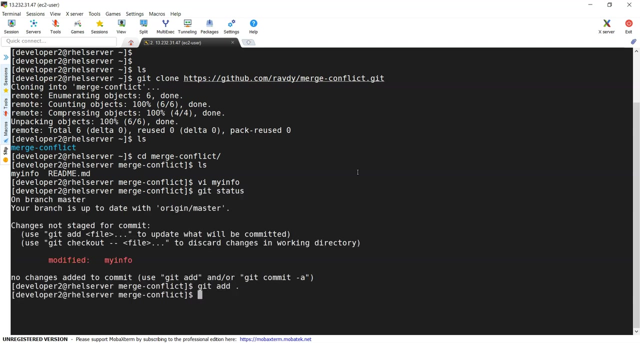 So, but he is working on master branch itself. He is not creating any separate branch. He edited my info and here developer two He has given and city name He might mentioned. Okay, So that's it. And git status: Git add dot. 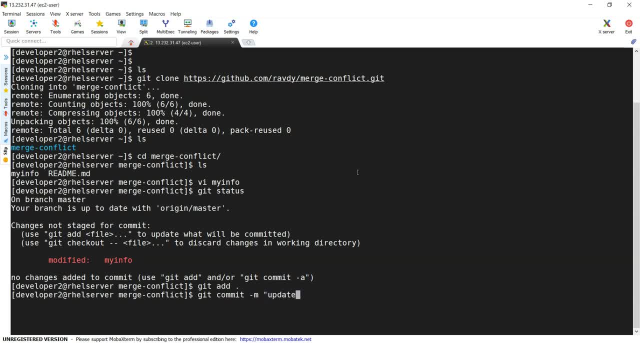 Git commit minus. m updated My info file Developer two. Okay, All right, So I have committed my changes onto master branch itself and git push Origin master. So I'm pushing my changes onto remote branch. It is asking for user name. 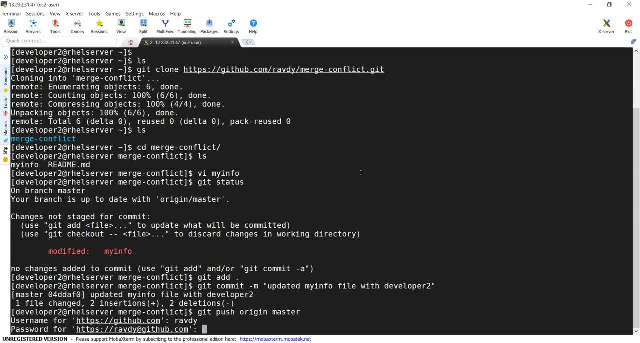 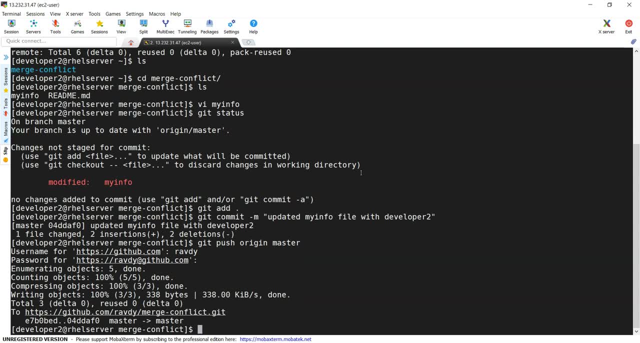 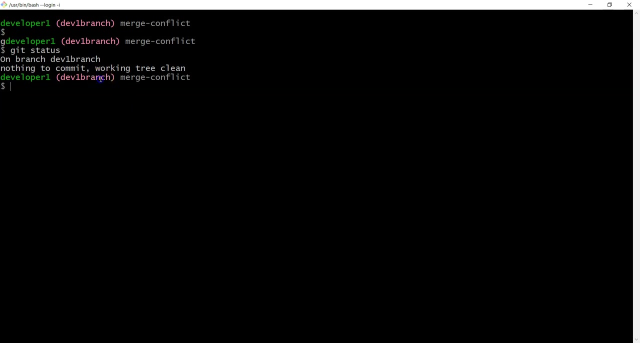 So revdy and I have given my password, Okay, So what happened in this situation is developer one and developer two. Both guys has pulled the same code and they updated the same file and same lines of code. But developer one Has taken his code and he created a new branch and he updated his code on the new branch and he is yet to commit his changes onto master branch. 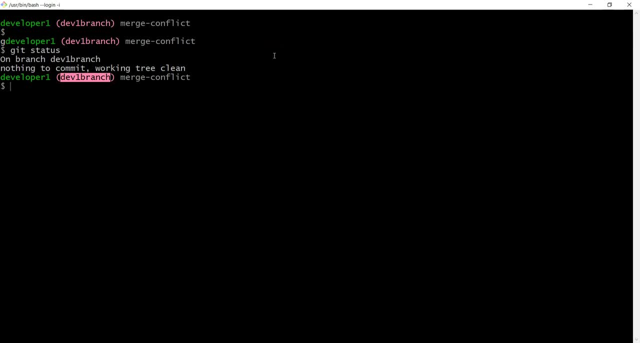 Once it goes to the master branch, from master branch to, he is going to push it into remote branch Meantime. developer two observed that Okay, There is some problems. So he has cloned the repository and he committed his changes into the remote repository. 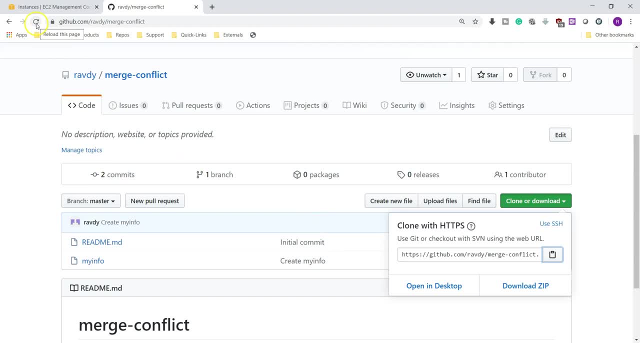 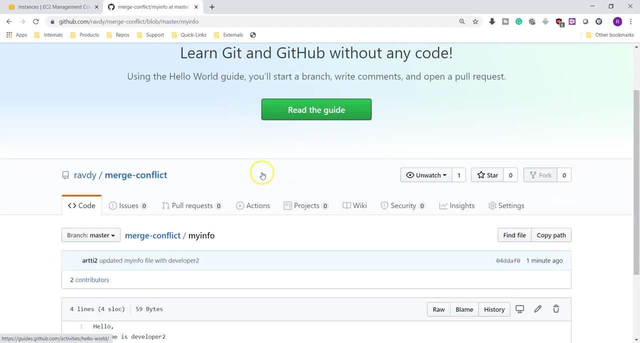 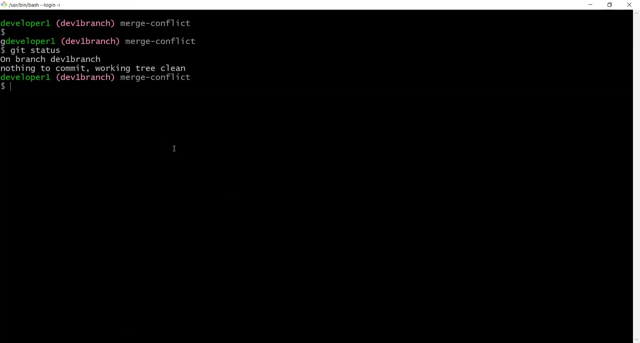 Now, currently it is two commits, but developer two already committed his changes. So it is going to update my info file and the three commits it came and if you see my info, it is already updated. Okay, Now developer one: he want to push his changes as well. right, 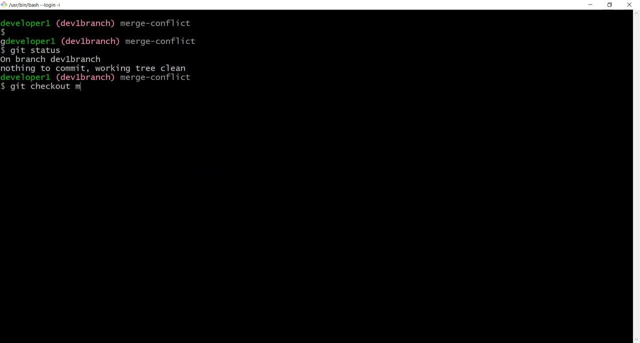 So he is switching back git checkout master. so he is going back to master and before pushing his changes he want to pull the code. Maybe he took some longer time and a few other developers might be updated the same repository. So due to that he thought that let me clone the repository. then let me merge my changes to the dev one branch to master branch. 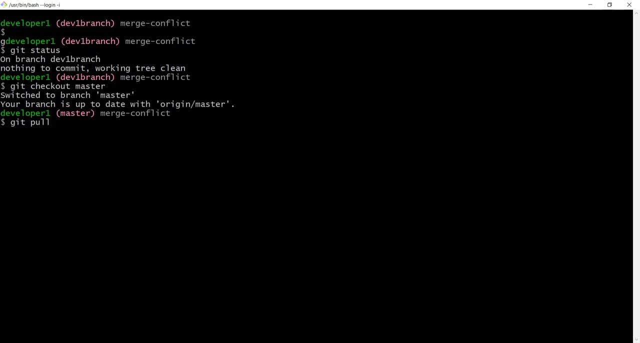 So git pull. so git pull is a command to clone the- sorry, pull the repository. So you can see here there were some changes and it pulled those changes. in my info file there are four changes: two lines added and two lines are deleted. Okay, anyway, he got latest code into the master branch at this moment. 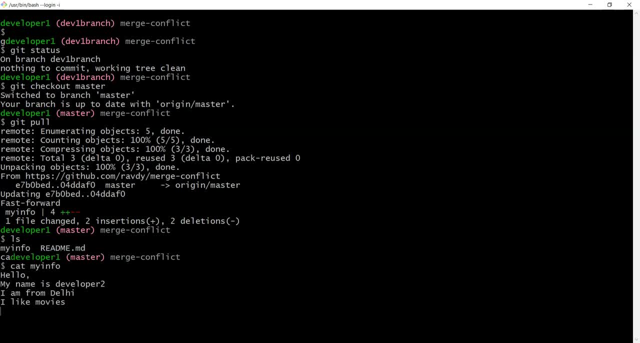 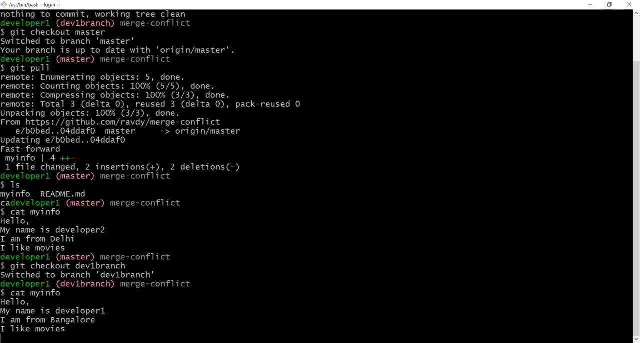 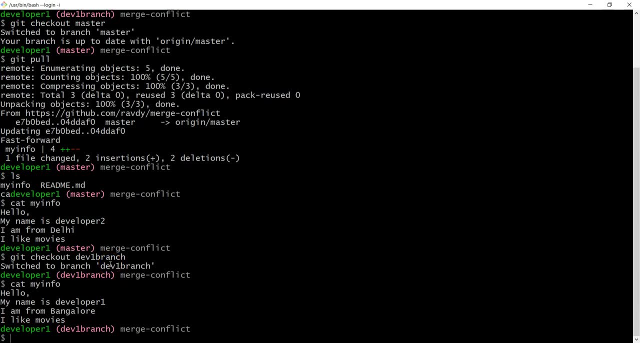 And if I open my info file over here so you can see that developer branch changes. Okay, now I would like to commit my changes onto the master branch. Usually, whenever you want to commit your changes, you should go to the destination. So if I go to the destination branch, in our case I want to commit my changes from dev one branch to master branch. 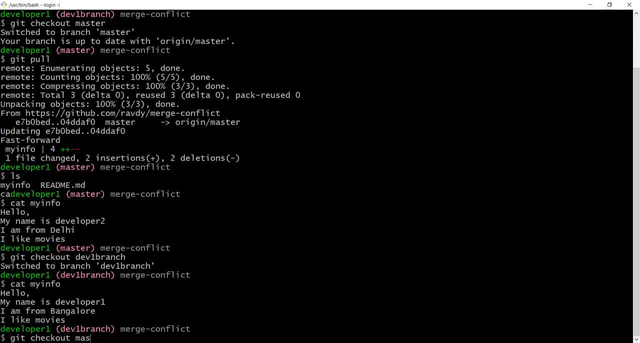 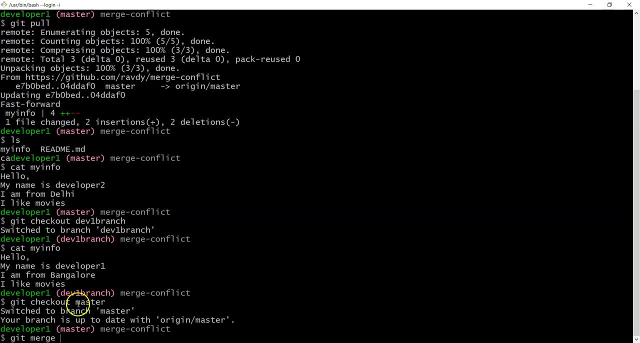 So switch back to master branch again. git checkout, master and merge your changes. So git merge and your branch name. So I want to merge the changes. whatever is there in the dev branch, one to master branch. Okay, you need not to specify the destination. 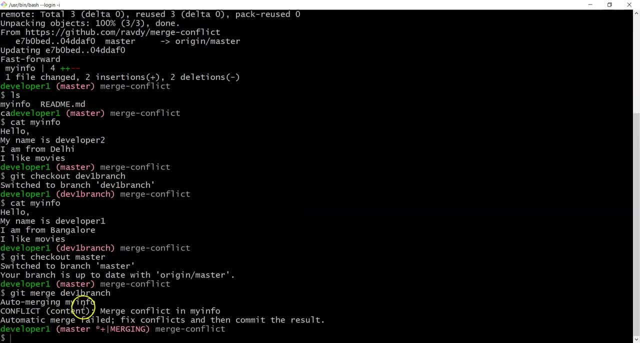 So if you do this one now, you can see here Auto merging my info. there is some problem with the my info. it is trying to auto merge the changes but conflict. there were some conflicts in the my info file. we need to fix those conflicts. that is what it is saying. 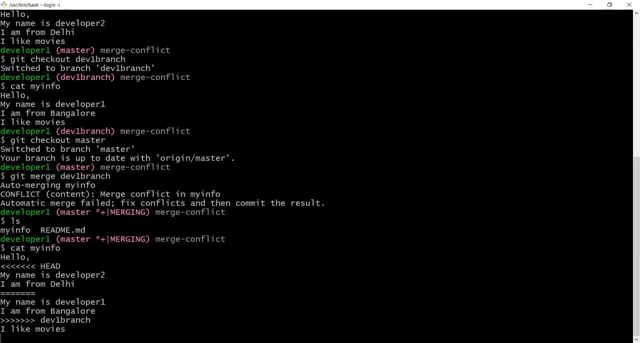 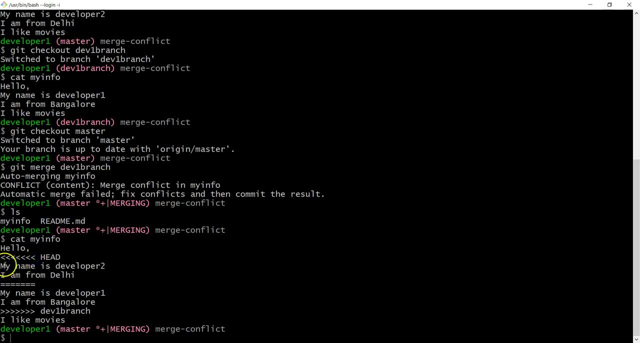 LS, if I open my info file cat, my info you can see here: your file has been updated and it has given the header nothing. but what is? the changes are same in the both the files you can see here. hello, there is no conflict. First line and last line also, I like movies, but remaining two lines. there is a conflict. that, okay, my name is developer two and I am. I am from Delhi, and same way. here also there is a conflict. 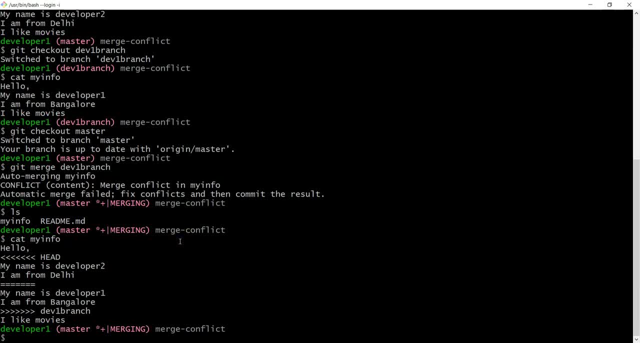 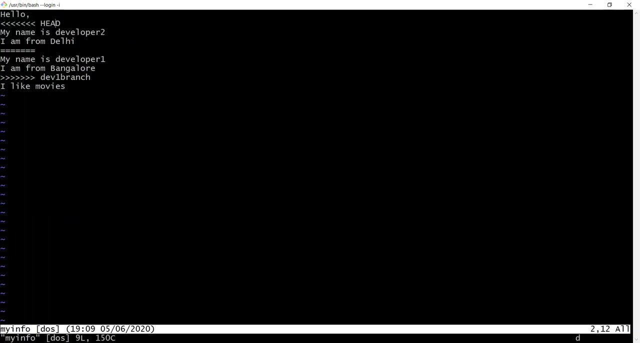 So now, usually what will happen in the real world? that group of people who has created conflicts or who has updated that code? they sit together and they discuss which changes are valid to fix this particular issue And then they update the code According to Their discussions and they push the changes. so in our case, developer one and developer two- sorry- sat together and discussed and come to a conclusion that, okay, let's keep the name as a developer one and keep the city from Delhi. so, like that, they have taken a decision and my info and we are updating according to the same discussion. so 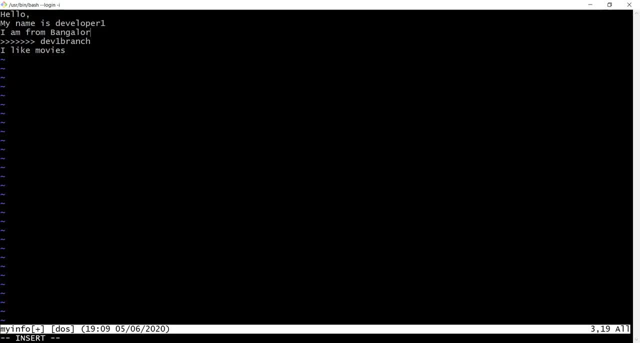 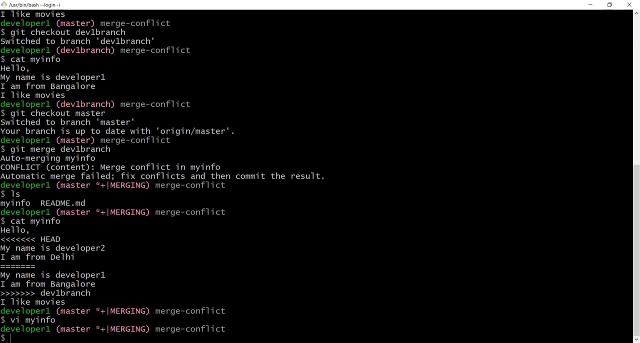 My name is a developer one and instead of My name is Sorry. I'm from Bangalore, I'm giving, I am from Delhi and remove this one also. okay, there are few tools which will help you to do this one, but usually this is how we do. 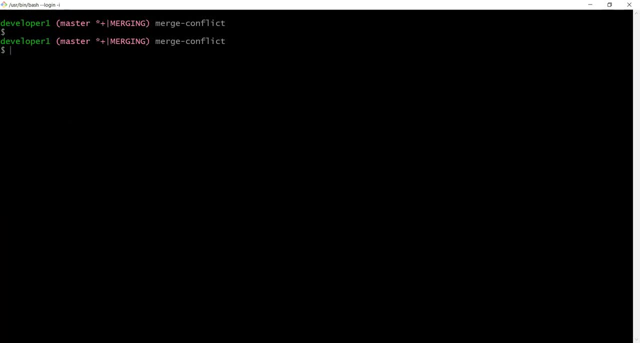 Okay if it is a smaller code. if there is a lengthy code, maybe you can use some third party tools. okay, get status. if you see now. so we have updated our file. now get status. if I check, sorry, now get add. Okay. next get commit minus cm. 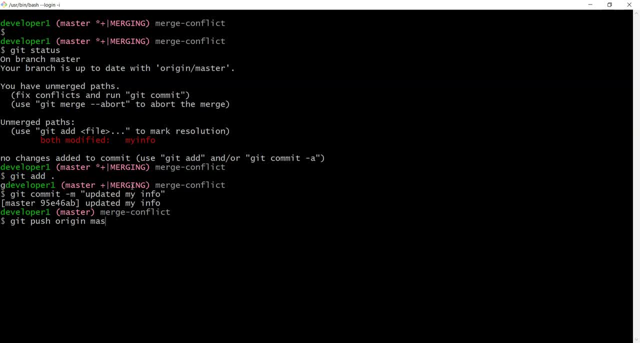 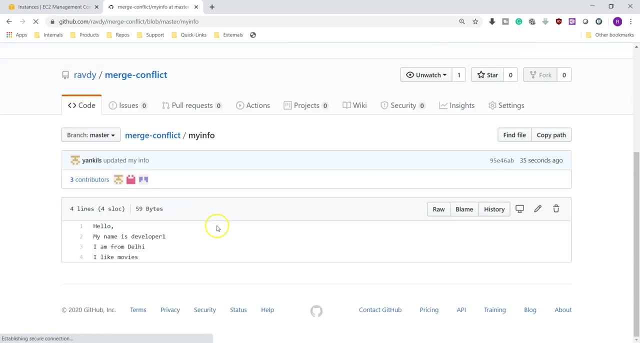 Okay, now get push origin master. okay, in master branch we are pushing our changes. Okay, my changes got pushed into my repository. if I go here and if I refresh it And the new changes has been updated, my name is developer one and I am from Delhi. okay, so this is how we get our changes. 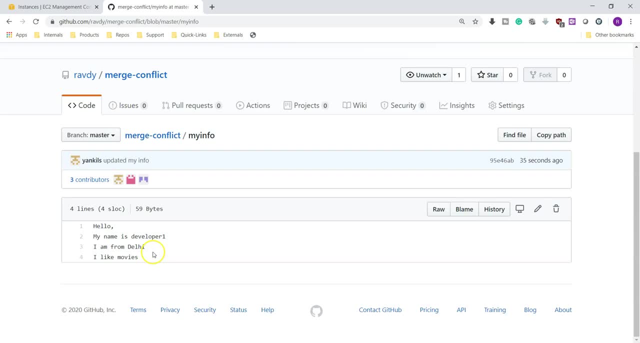